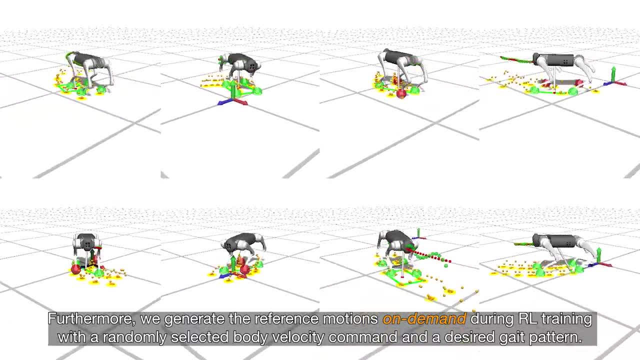 we generate the reference motions on-demand. RL training uses a randomly selected body velocity command and a desired gait pattern. 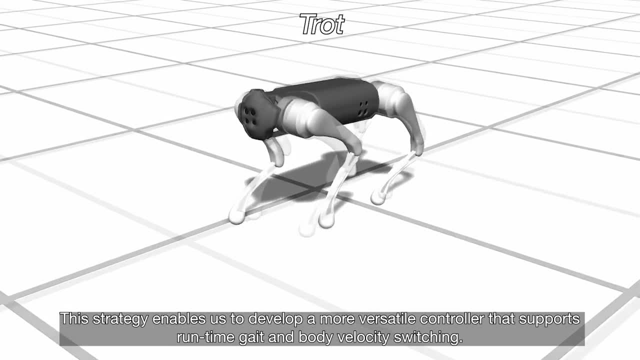 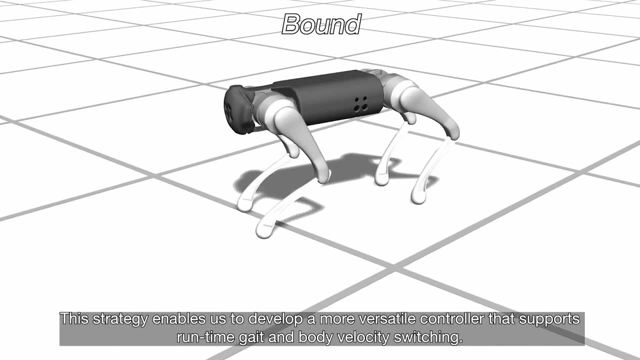 This strategy enables us to develop a more versatile controller that supports runtime gait and body velocity switching. 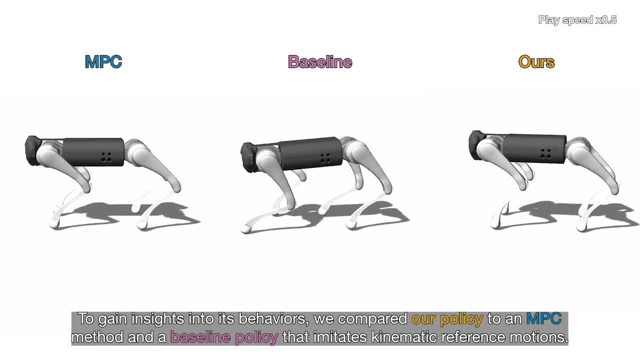 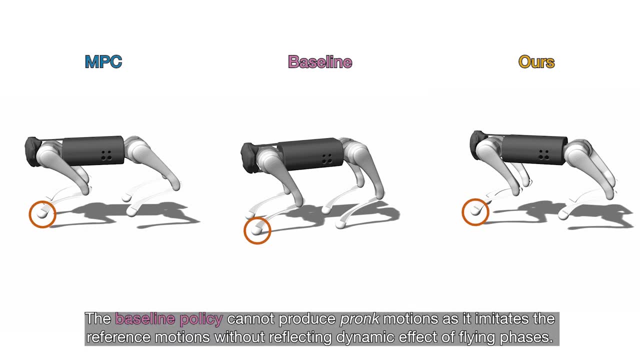 To gain insights into its behaviors, we compared our policy to an MPC method and a baseline policy that imitates kinematic reference motions. The baseline policy cannot produce prong motions as it imitates the reference motions without reflecting dynamic effect of flying phases. 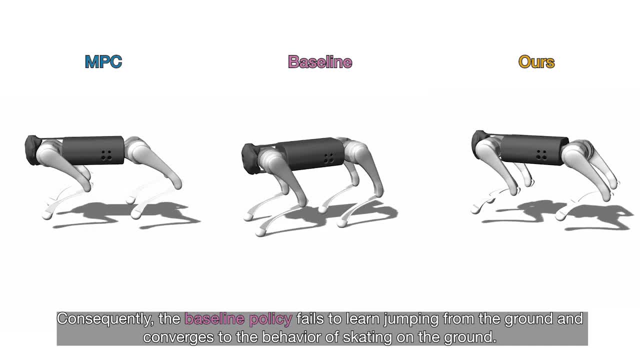 Consequently, the baseline policy fails to learn jumping from the ground and converges to the behavior of skating on the ground. This highlights the importance of addressing the dynamic effect in generating reference motions. 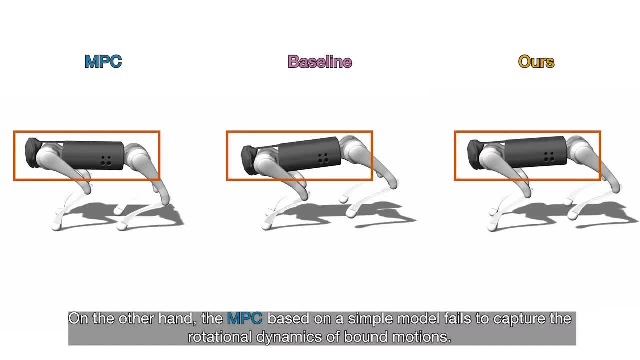 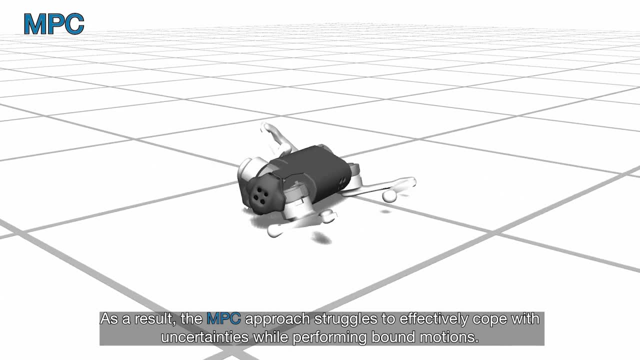 On the other hand, the MPC based on a simple model fails to capture the rotational dynamics of bound motions. As a result, the MPC approach struggles to effectively cope with uncertainties while performing bound motions. 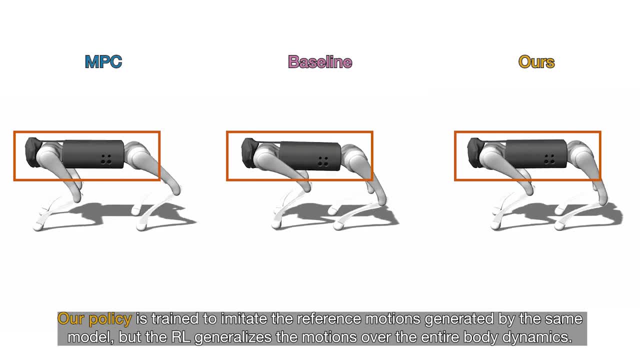 Our policy is trained to imitate the reference motions generated by the same model, but the RL generalizes the motions over the entire body dynamics. 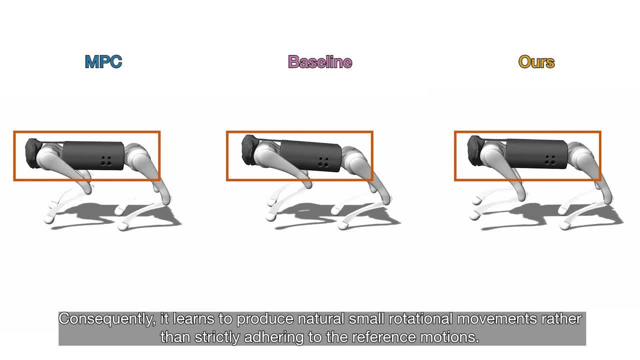 Consequently, it learns to produce natural small rotational movements rather than strictly adhering to the reference motions. In the second experiment, we assess the robustness of our policy in reducing the dynamic effect of flying phases. 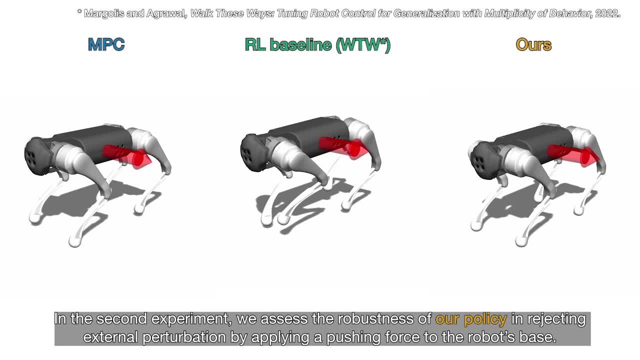 In the third experiment, we train our policy in rejecting external perturbation by applying a pushing force to the robot's base. 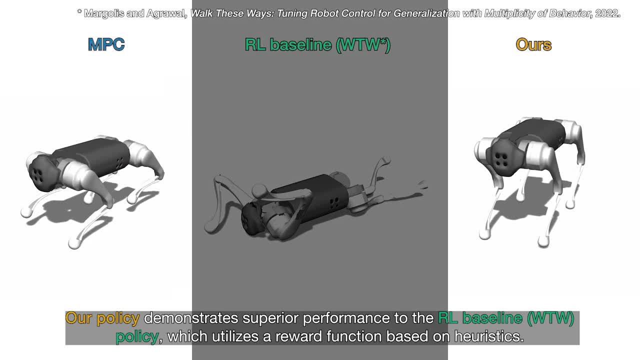 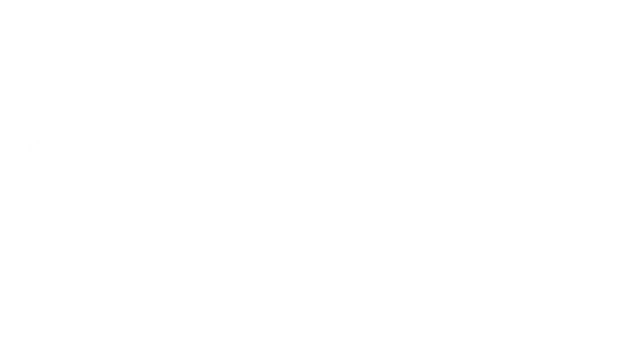 Our policy demonstrates superior performance to the RL baseline, namely walk-these-ways policy, which utilizes a reward function based on heuristics. 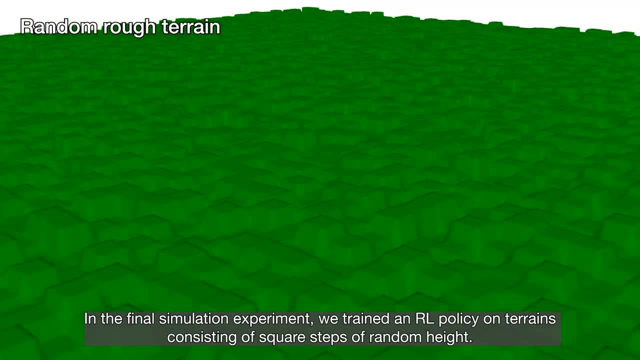 In the final simulation experiment, we trained an RL policy on terrains consisting of square steps of random height.